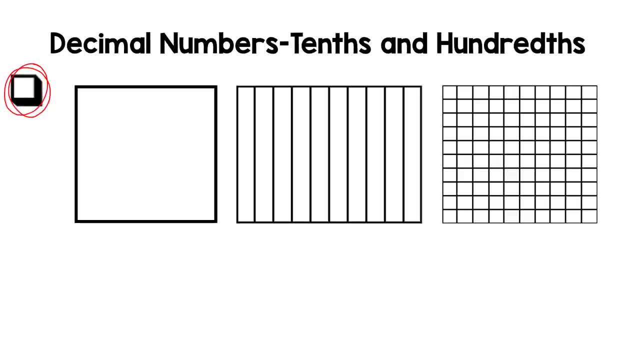 with you about earlier. This is also called a unit. Now this is one whole square. It's not broken up into any parts. Imagine kind of like one whole cake, one whole brownie pan. Now here is one whole square, but this one is actually split up into 10 equal pieces and we represent that as 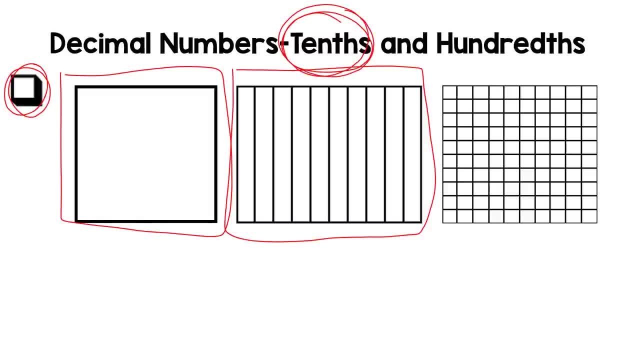 tenths. That's why it's called a unit. So we're going to take each of these and we're going to break them up into smaller parts. Now, we're going to take each of these and we're going to talk about the tenths place, and it is also represented in fractions, with a denominator of. 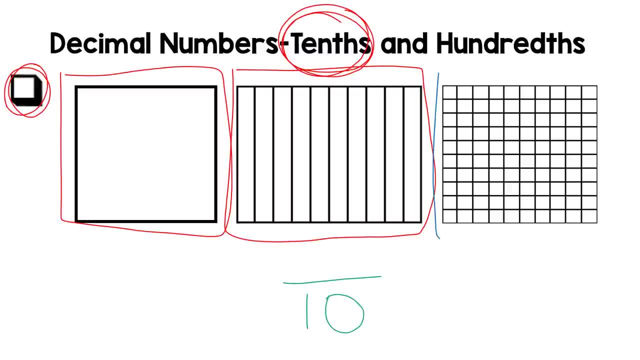 10. This square is one whole square, but it is split up into 100 equal pieces. That's why it's called hundredths, and in fractions, the denominator is 100.. 100 equal parts. So now the place value that we're all we're going to be using as we discuss tenths and hundredths is going to be: 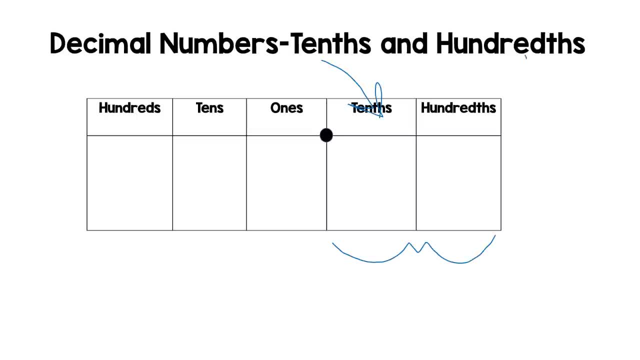 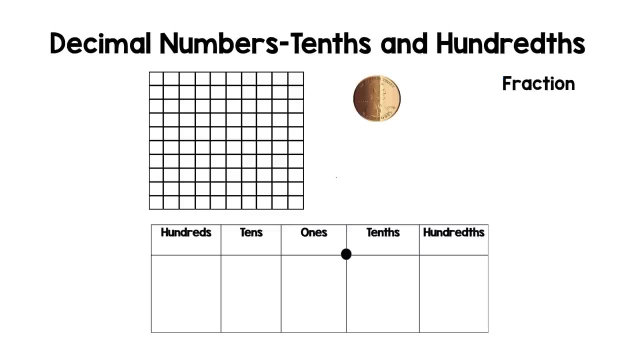 here. This is the tenths place, This is the hundredths place, and here, separating the ones place and the tenths place, is our decimal. We don't call it a dot or a point, It is a decimal. So let's put our decimal numbers in actions. Here you have a decimal grid. It has 100 equal pieces. 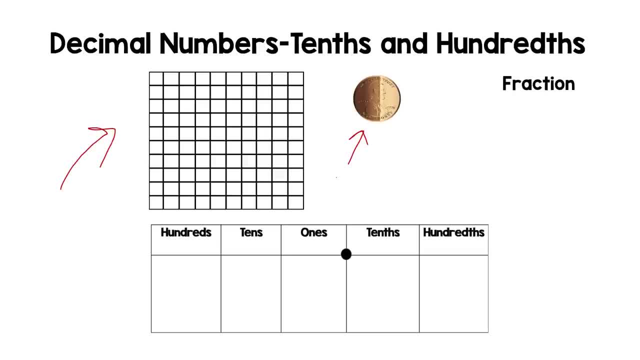 I have a penny which represents one out of 100 cents of a dollar, So I'm going to represent this penny on the grid. I'm going to put a penny on the grid and I'm going to put a penny on the grid. This is worth only one cent, so I will color in only one part here. 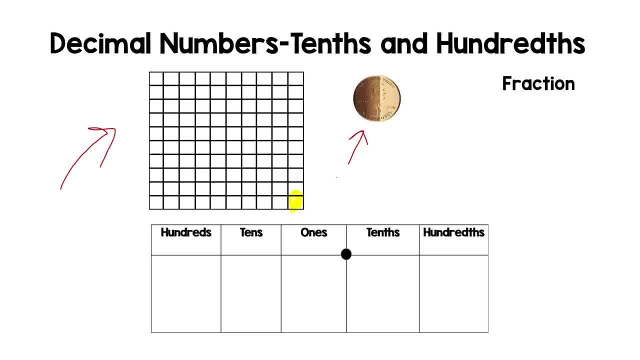 Try and get it thick enough there. So we'll say that that's one one hundredth of a dollar, and if I'm going to represent that on my place value chart, I have one hundredth, zero tenths and zero ones, and this is how I represent that number. 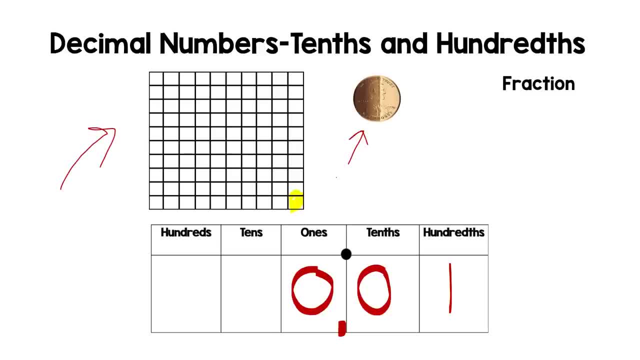 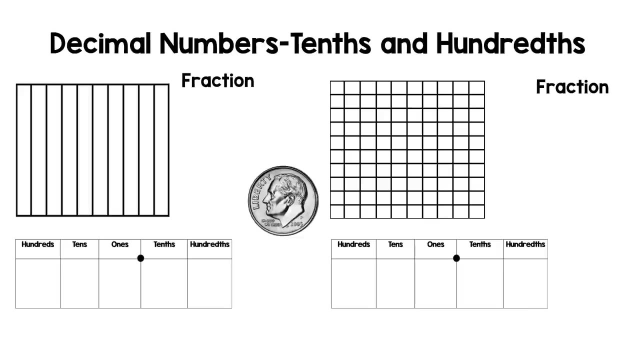 One hundredth. If I represent it as a fraction, I would put one out of one hundred is what a penny is equal to, That's hundredths. Now let's look at a dime. Now, a dime is special because a dime fits into a dollar ten times. but I can also represent it on the hundredths grid over here, as. 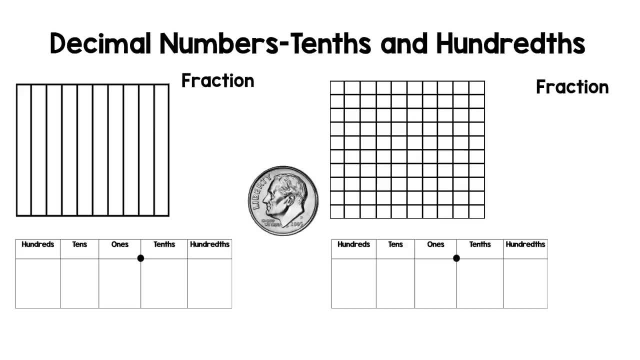 ten hundredths. So let's go ahead and shade in what we know. One dime is actually one tenth of a dollar, and if I shade it in one tenth I would shade it just like this, Not quite so neat, but you get the idea. And my fraction is one tenth of a dollar. I write. 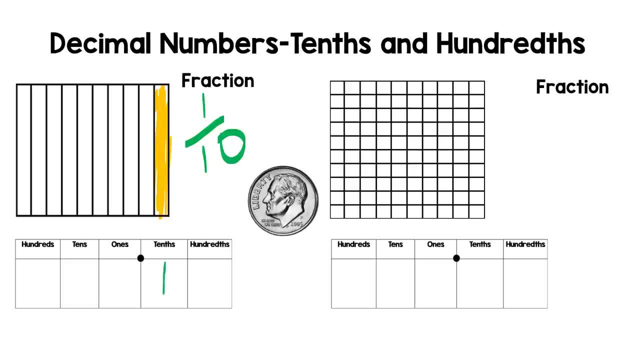 it in my place value chart as one tenth. I have zero ones and there is my decimal. That's how I write one tenth. Now, if I were to take this same dime and put it in this grid, I would shade ten parts, because a dime is. 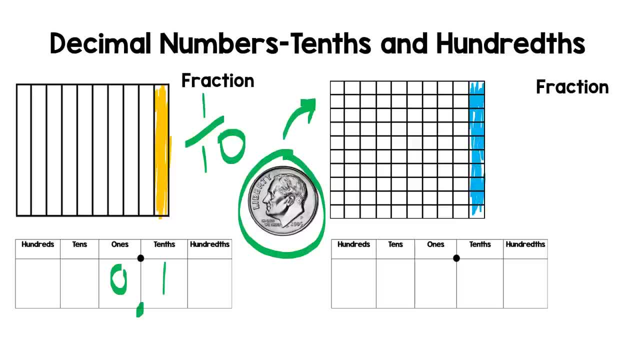 actually ten pennies, That'll be good enough, And I'm going to put this as ten out of one hundred, And if I were to write that on the place value chart, it's pretty much the same. I can have zero ones. my decimal 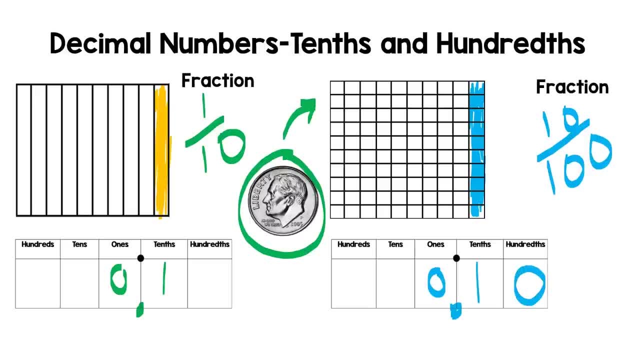 and ten out of one hundred. So, as you can see, on this one I have a zero in the hundredths place. In this one I have no zeros or anything in the hundreds place, It's just one tenth. but these are actually equivalent. They. 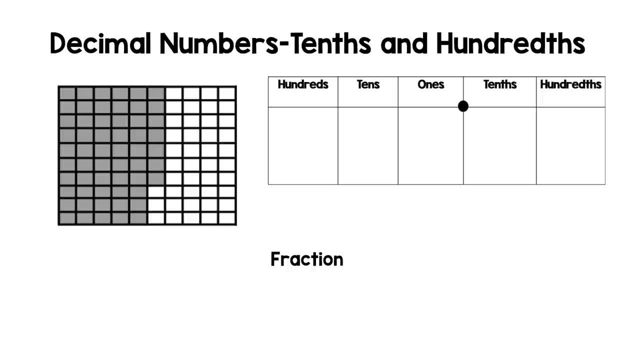 equal the same thing. Alright, so let's look at some actual decimal grids that have been shaded. So look at your decimal grid here. As you can see, this grid has part of it shaded. It's not one whole, but it's painted to the perfect color. This grid looks like its number one. 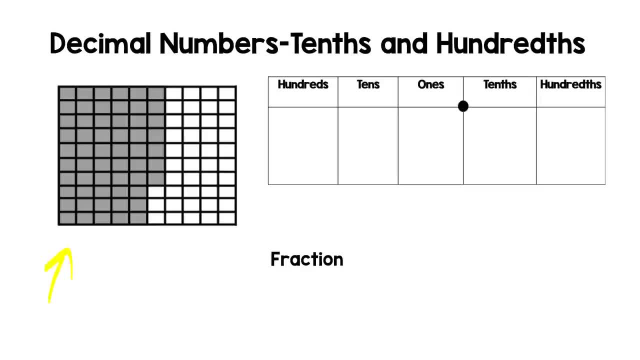 can see, this grid has part of it shaded. It's not one whole, but it's part. So I know that in my ones place I'm going to have a zero because there is not one whole shaded and there is my decimal. So when I tell my students to count, I say go ahead and count the columns. It's easier to count that. 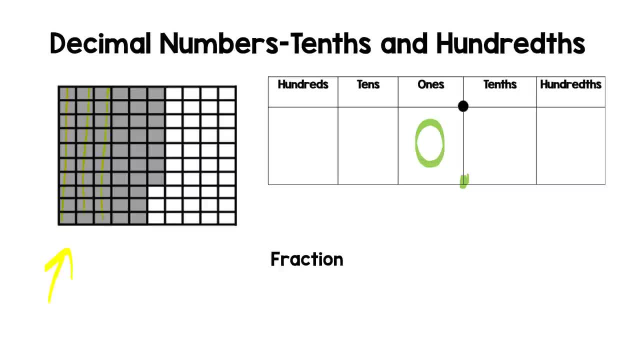 way. So this is 10,, 20,, 30,, 40,, 50, and now we'll count the ones 1, 2, 3, 4,, 5,, 6, 7.. So I know that.